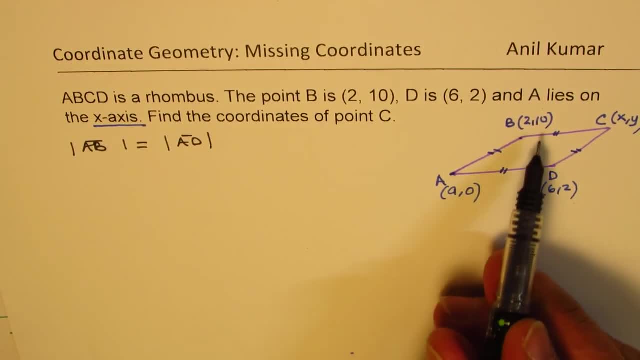 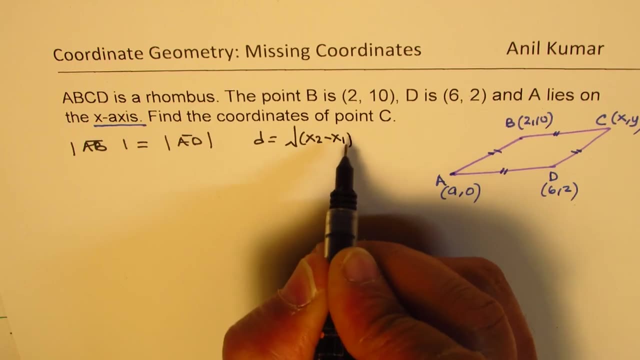 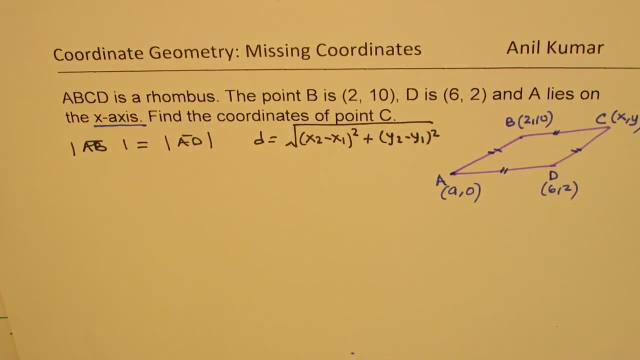 So that should give us coordinates of A Length. is you know the formula, distance formula, which is square root of x2 minus x1, whole square, plus y2 minus y1 whole square? So that formula can be used, We could actually square and then compare also. So no need to square root, okay. 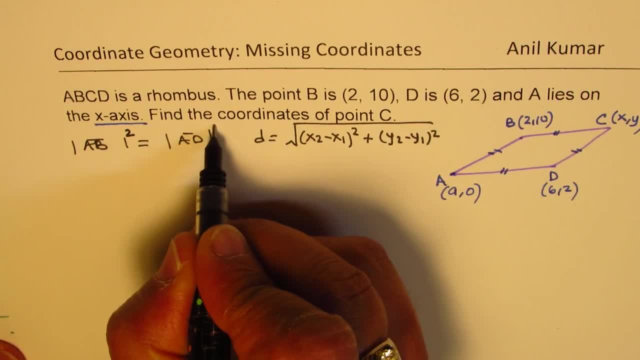 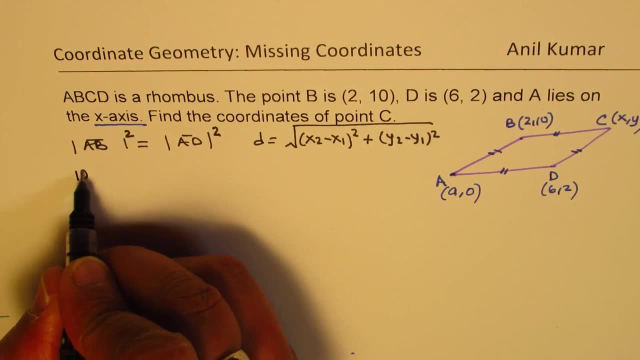 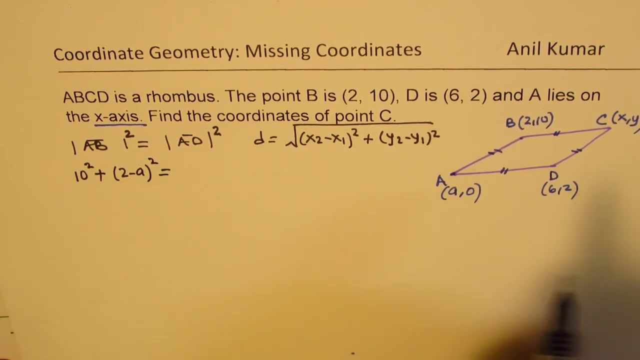 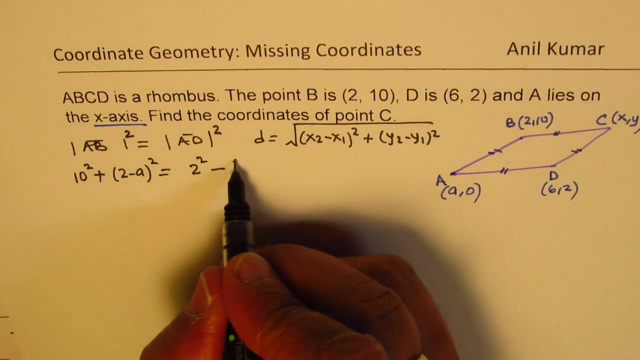 So we'll say that the length squares are also equal, correct, That's the whole. that's better. So A to B length will be 10 minus 0, which is 10 square plus 2 minus A whole square is equal to A to D, which is 2 minus 0, which is 2 square minus 6 minus A whole square. 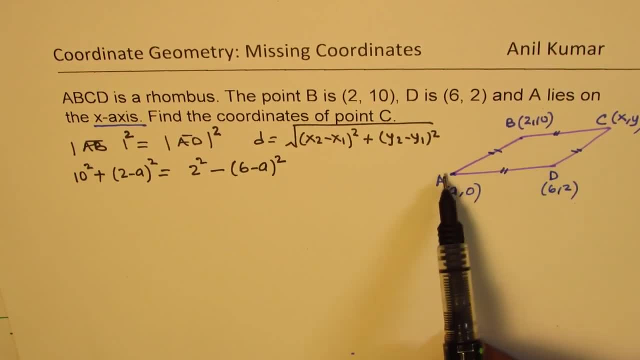 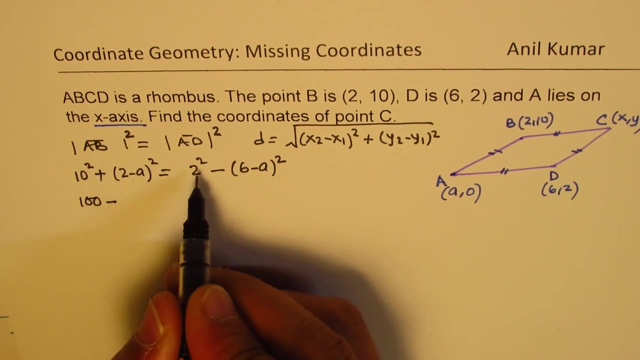 So we get this. So we are equating these two lengths square of these, these two lengths. right Now, to solve this, easiest method will be: we'll use difference of square. See how We have 10 square, which is 100, minus. 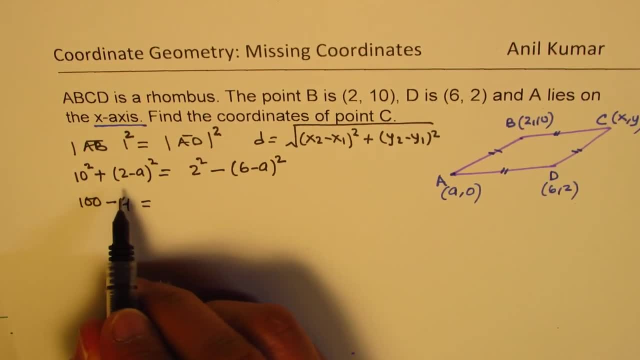 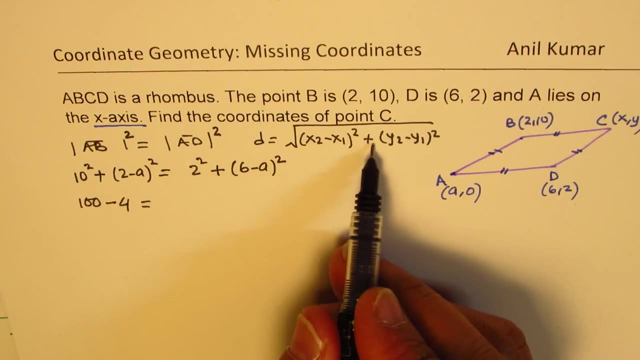 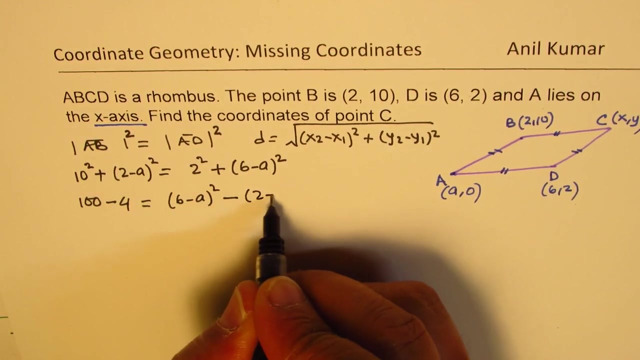 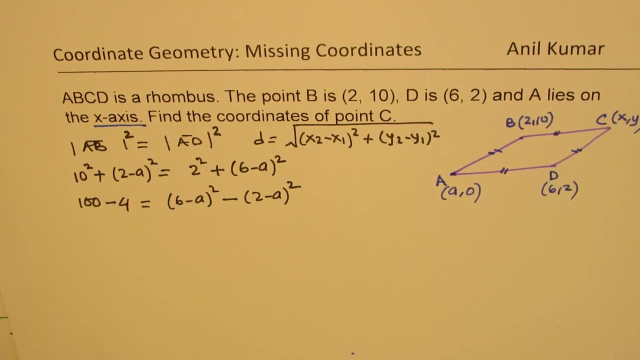 Let's bring 2 square here, which is 4, equals to: well, this is plus, not minus A plus right? So we have 6 minus A whole square, minus 2 minus A whole square, correct? So we just rearrange: took 2 minus A to the right side and 2 square to the left side. 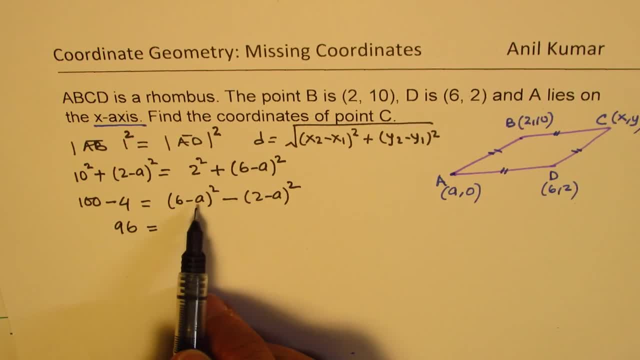 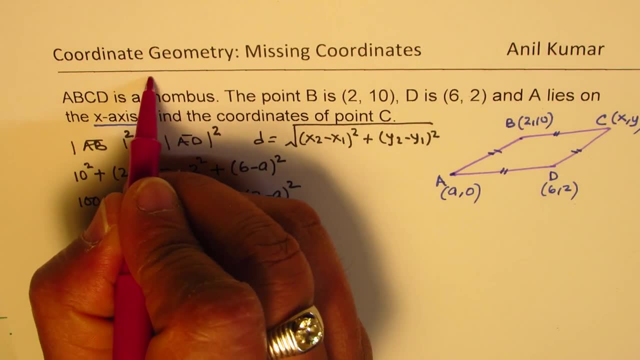 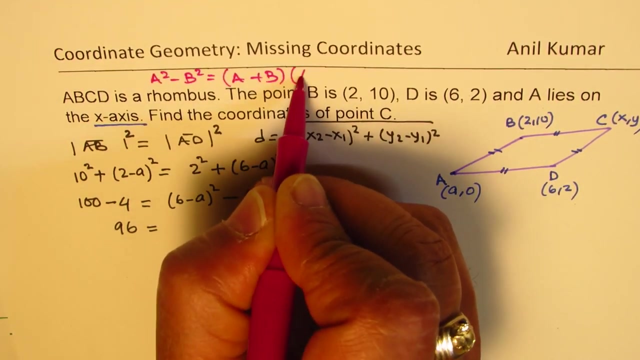 100 minus 4 is 96.. And here we have difference of square. Now here's a very important formula which you should remember. If we have, you know, capital, A square minus B square, we could factor this as A plus B times A minus B, correct? 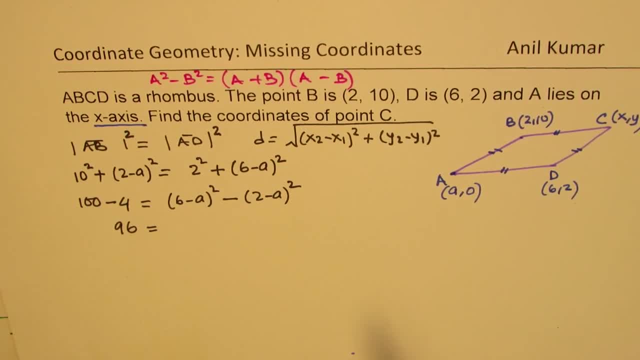 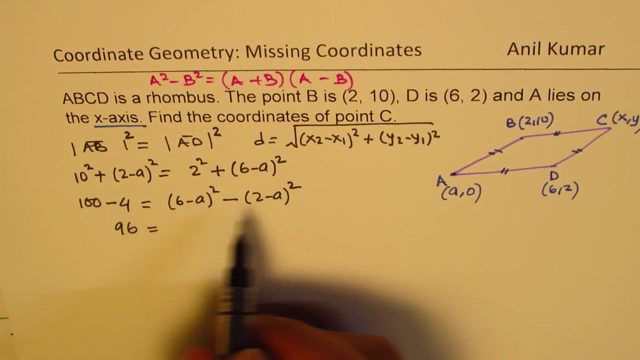 So instead of expanding and simplifying, I'll actually factor and then find: okay, It'll be simpler for us. So what we get here is 6 minus A whole square minus 2 minus A whole square, or we could just expand it also, but factoring is better. 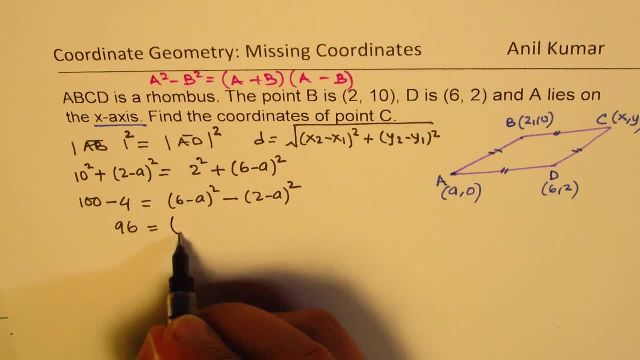 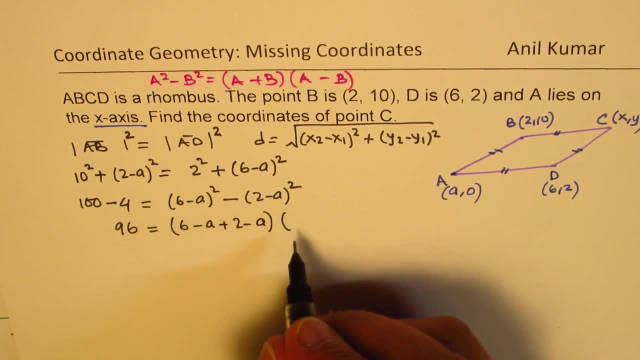 So I'll adopt this factoring technique. So A plus B means 6 minus A plus 2 minus A. times A minus B means 6 minus A minus 2 plus A. okay, So that is what it is. So we can say: 96 equals 2.. 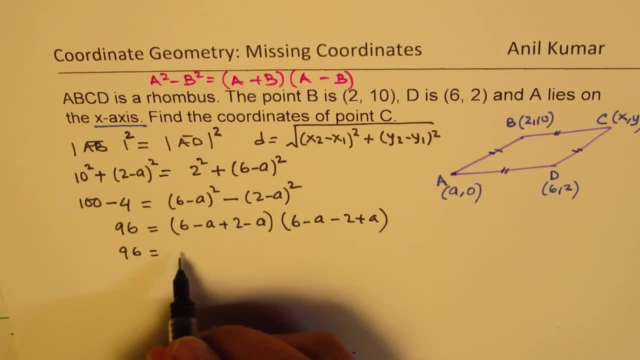 6 minus A. minus is minus 2A, 6 plus 2 is 8. We get 8 minus 2A. Here. we get: 6 minus 2 is 4. And minus A plus A is 0. So we get just 4.. 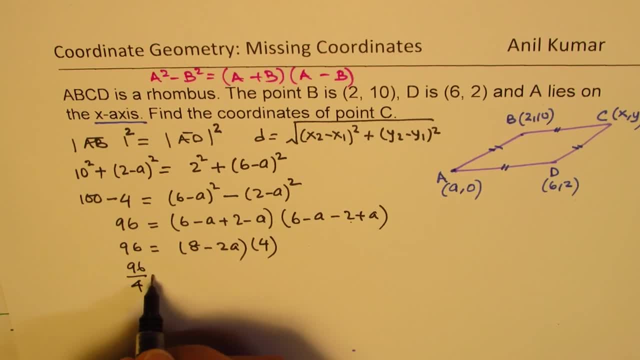 So we can write this as: 96 divided by 4 equals to 8 minus 2A, 96 divided by 4.. 4 times 2 is 8, 24, right? So now we can solve for: 2A equals to 8 minus. 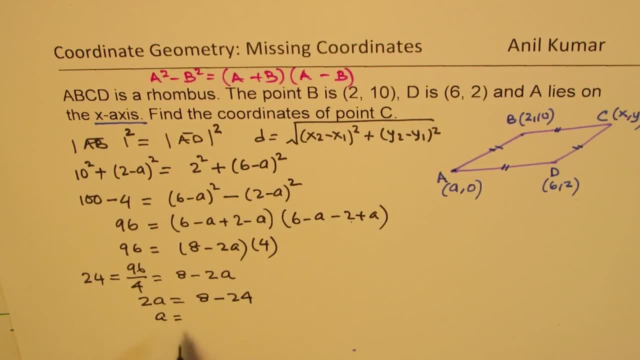 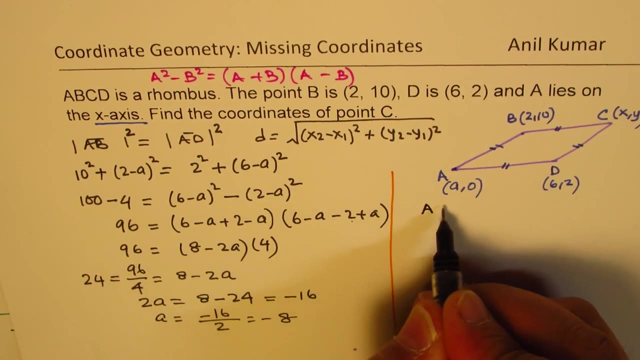 minus 24.. So that gives us A as equal to 8 minus 24 is minus 16.. So minus 16 by 2,, which is minus 8. So we get the value of A as minus 8.. So the coordinates for A are minus 8,, 0, clear. 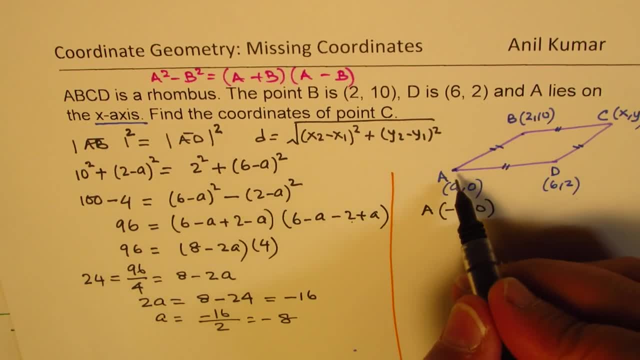 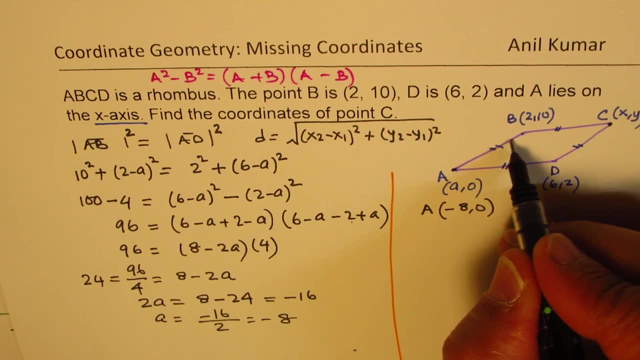 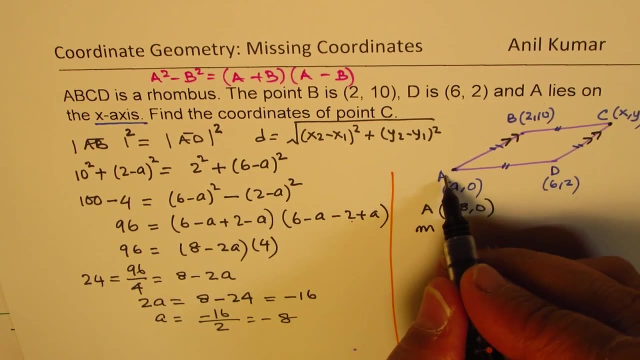 So we got coordinates of A. Now we need to find coordinates of C. Now we could use the, The concept of slope, since the slope is right, these two are parallel lines, correct? So we know the slope from A to B is same as slope from D to C. 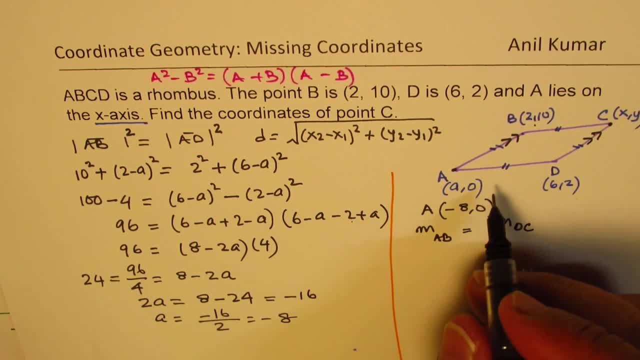 Slope from A to B is 10 minus 0, right, So it's just 10 minus 0.. And the Y values and X values are 2 minus 8, which is minus 8.. So 2 minus minus 8.. 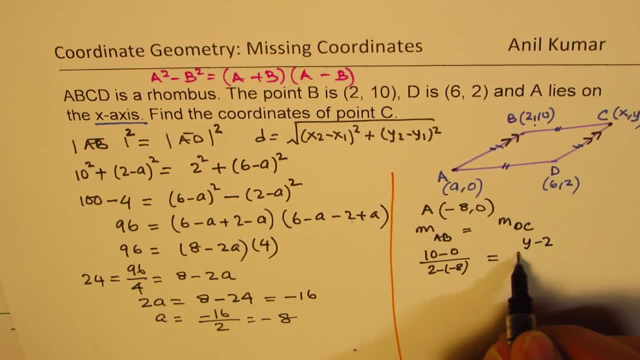 Slope from D to C is Y minus 2 over X minus 6.. Now this gives us 10 over 2. minus means 10 over 10, right. This becomes 10 equals to Y minus 2 over X minus 6, correct. 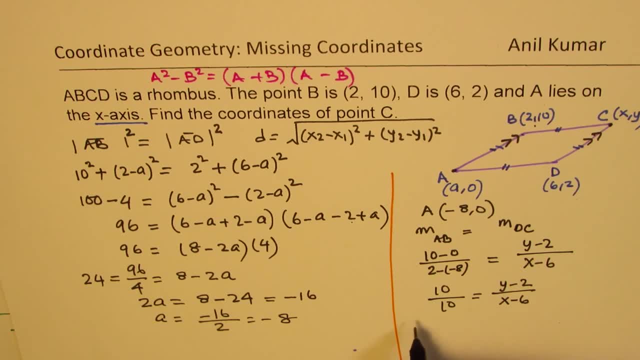 So we can equate separately Y minus 2 as 10.. So we get Y minus 2 equals to 10.. So Y is equal, Y minus 2 equals to 12.. And we have X minus 6 equals to 10.. 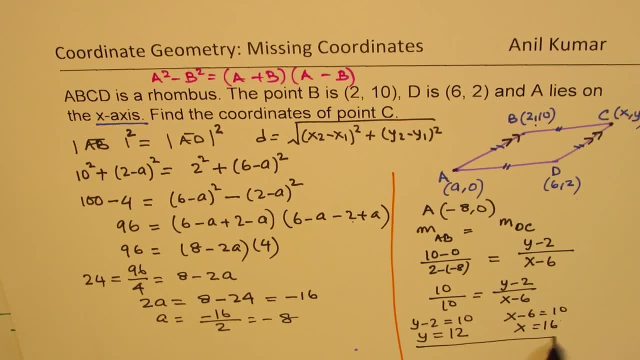 X equals to 16.. And that gives us the coordinate points of point C as 16 and 12, right? Do you see this idea? right? So that's a brilliant idea. We could always write this as 16, 12..